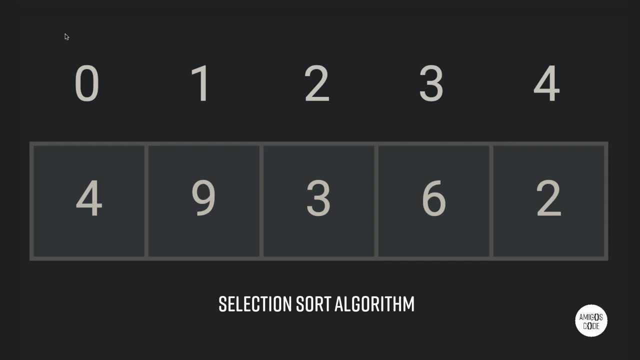 algorithm. So selection sort is one of these algorithms which is really simple for you to understand. And right here you see that I've got this array, So containing four, nine, three, six and two, And above you can see the actual indexes. So zero, one, two, three and four. So 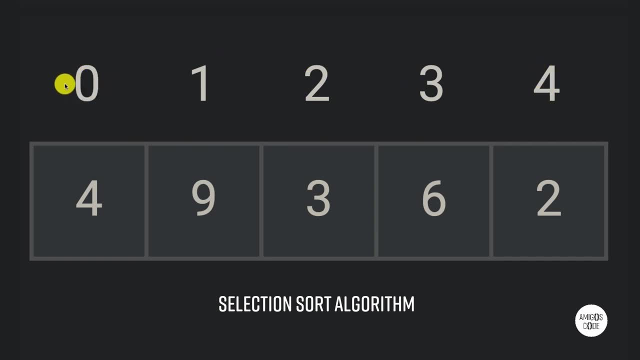 those are the actual positions for your array. So the way it works is as follows. So we're going to start from the beginning And what we're going to say is four, Right. So we're going to start with four and we're going to go till the end and try to find. 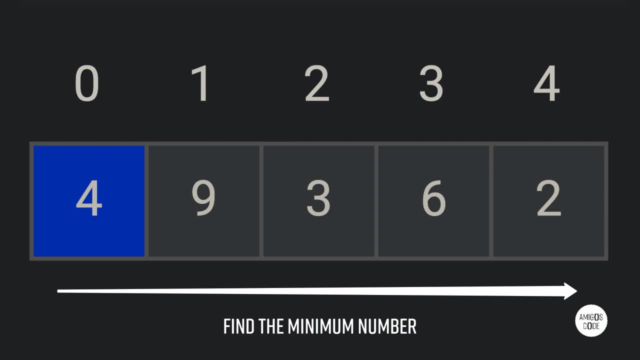 the minimum number from index zero to four. So is four less than nine? Yes, So four. So the minimum number is four less than three, No, Right. So three now becomes the minimum number, And now we say it's three less than six, Yes, 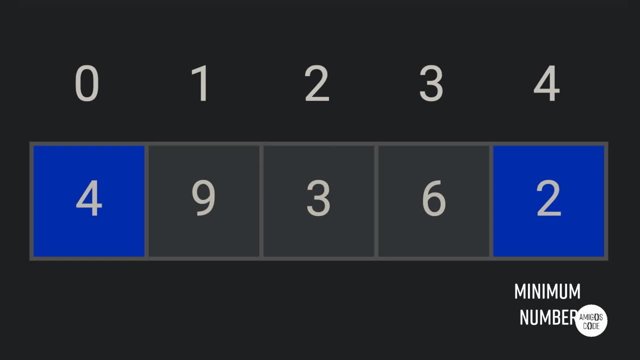 It's three less than two, No. So two now is the minimum number right in this array. So what we're going to do now is simply swap two and four, just like that. So you see that we've swapped two and four. Now two is in the right position. So now we're going to carry on from one, So index one. 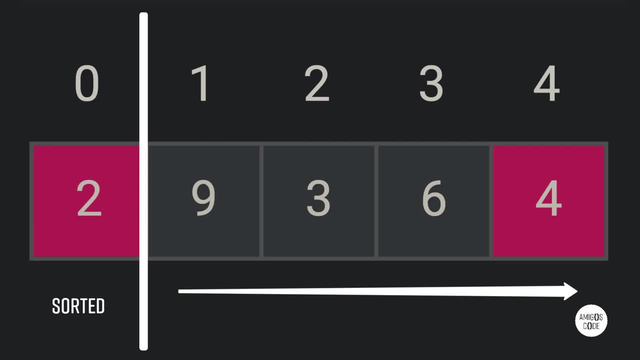 to four And we're going to repeat the exact same process. So we'll start with nine. Let's find the minimum number. So we know that three is less than nine, So three now becomes the minimum number And we're going to carry on. So six is bigger than three And four is also bigger than three. 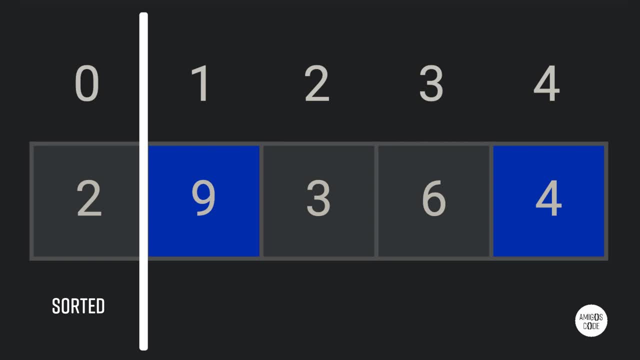 So three is a minimum number And we're going to swap three with nine. So right here. So we swap three with nine. Now two, three are sorted. We're going to start from index two, Right, And we're going to find the minimum number. 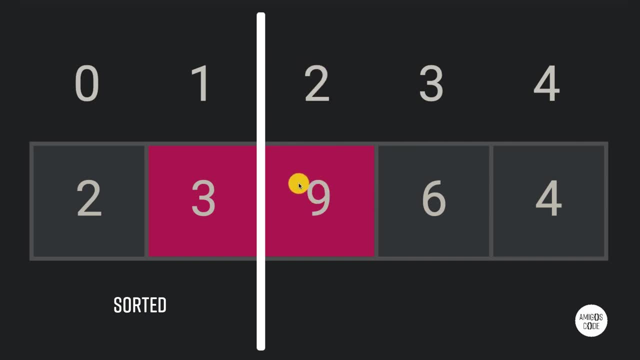 So right here. So from two to four, we're going to find the minimum number. So you can see that the minimum number is four. So let's play the animation. So there we go. We found four. Four is less than six And we're going to swap four with nine. Now let's carry on Six. 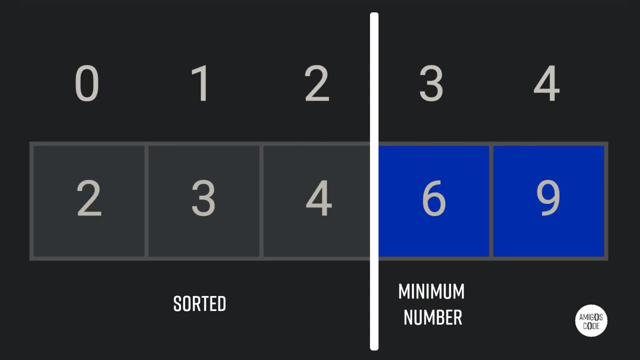 is six, The minimum number. Yes, We're going to now leave six in the exact same position, Right, And there we go. So we now sorted the array. So it's as simple as this. Now let's go ahead and learn how to put this into code, Right? So for this video, I'm going to be using Python. 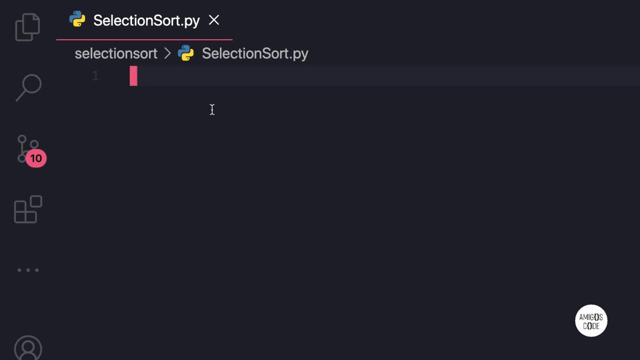 And in the previous video I've used Java, JavaScript and Python to demonstrate that language is just a tool. So if you want me to use a different language for the next video, go ahead and suggest which programming language you want me to use to. 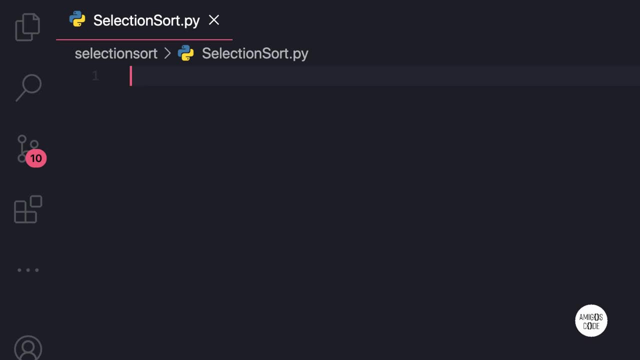 demonstrate the actual algorithm. So right here, let's go ahead and simply create the actual numbers, Right? So equals two, and then this array and the numbers were these ones. So four, nine, three, six and two. Now what we're going to do is pretty much just create a for loop. 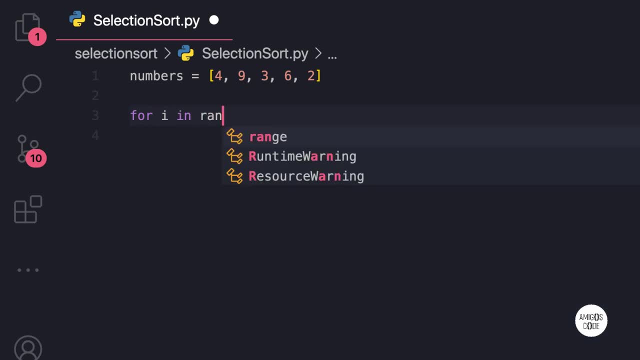 And we're going to say for I, and then in, and then range, and then the length of numbers- Right Numbers, just like that- And then column there. Now, what we're going to do is simply start from the beginning, right, And we need to initiate our minimum number. So I'm going to say: 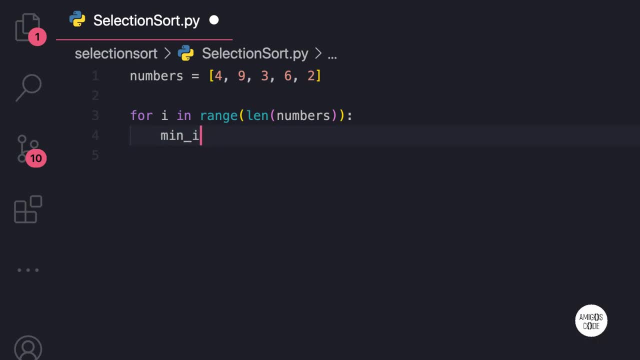 that the minimum index, Right, So index is equal to I to begin with. Next, what we're going to do is say four, Right, So now four J, and then range, And right here we're going to start from I plus one And we're going to go. 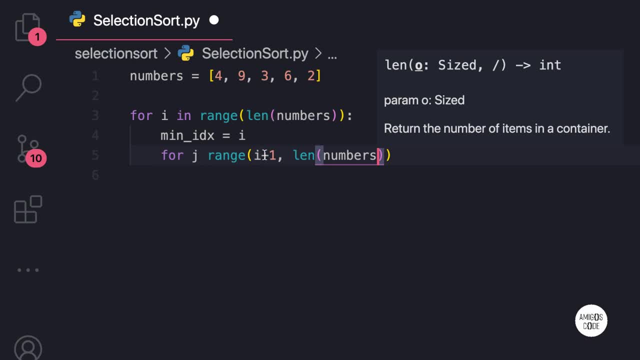 through the length of numbers. So the reason why I'm say I plus one is because I want to compare. So initially this will be four, But the J right. I want to start from this number right here. So J will start from I plus one. 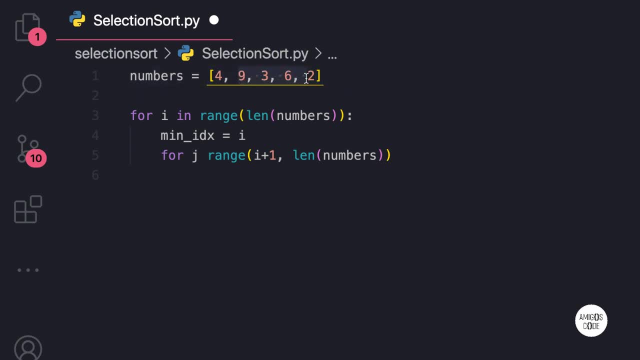 Right, So right here. And then the next time it goes to the loop it will start right here. The next time- Oops, Actually right here And the next time right here. So basically, it's the exact same example I've showed you in the animation And what we're going to. 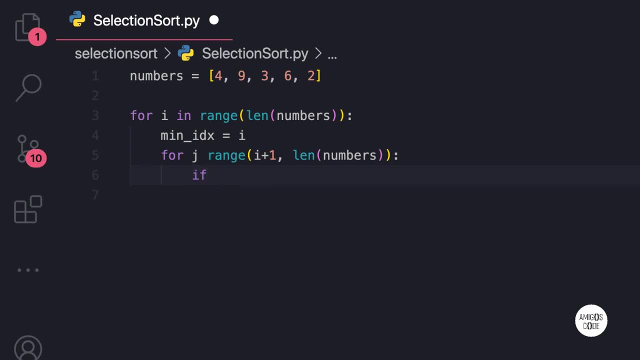 do is simply say if Right, So. we want to say if the numbers Right, So, and guess what? So the numbers at index J Right? So if this is less than the numbers, and then right here, guess what. The minimum. 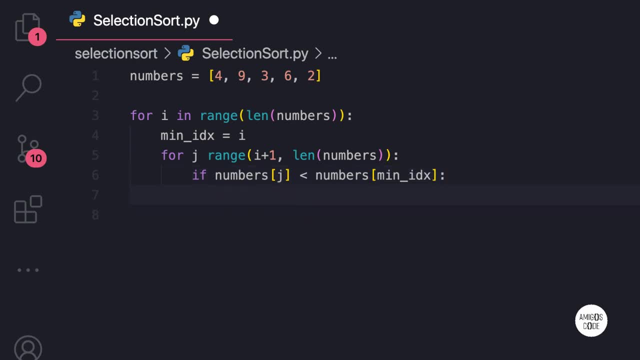 index. So if this is the case, we have a new lowest number. So I'm going to say mean, and then index equals two, and then J, Right. So now that we found the minimum index, remember, all we have to do is simply. 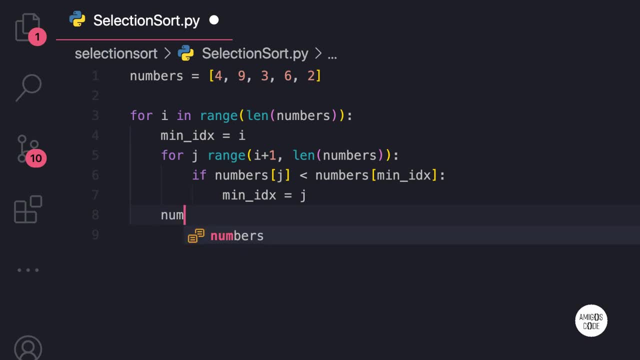 swap the numbers. So I'm going to say numbers and then I Right, So I will be from zero, So zero. So I want to swap the zero index, So four in this case, with two Right, Because two will be initially the lowest. 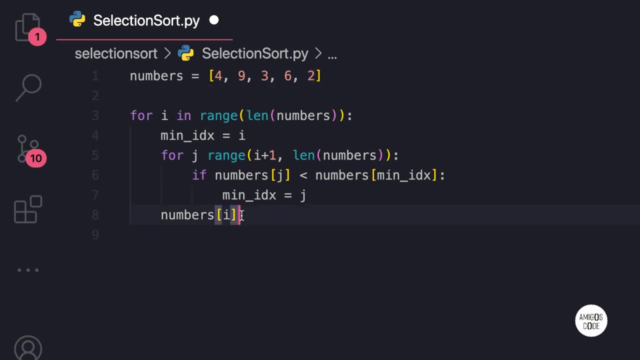 number in this array, Right. So I want to swap I and then numbers and then right here mean index equals two, and then numbers mean index And finally numbers and then I. So this is how you swap numbers in Python. So the reason: 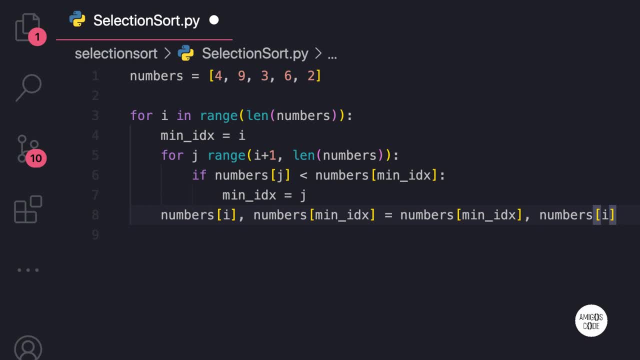 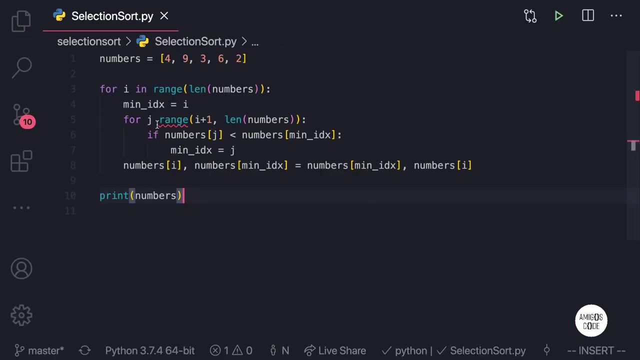 why I'm choosing Python is because Python is very simple to you to read and reason about. So this is the actual algorithm. So let's now go ahead and simply say print and then the actual numbers. There we go, And if I save this, we've got an error right. 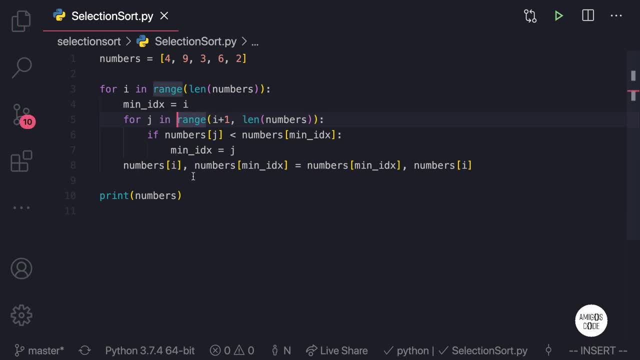 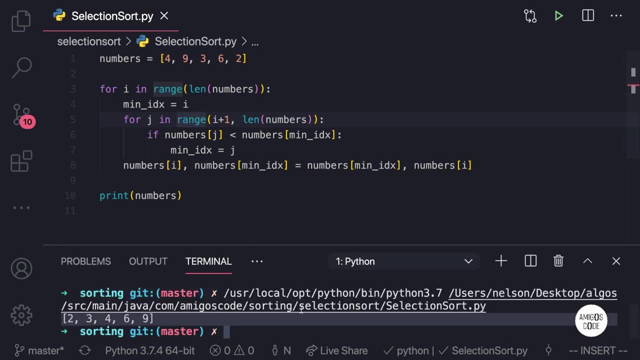 here, So this should be in Right, And then save again. There we go Now, if I run, and there we go, So you can see that we have the array sorted. So four. So let me put this bigger, So you see. 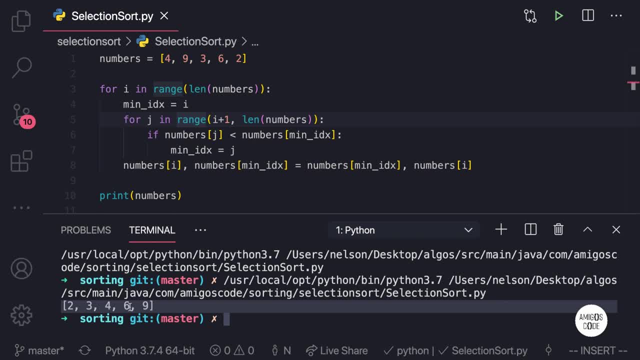 So here two, three, four, six and nine, And this is pretty much everything about the selection sort. Now, selection sort is not the quickest algorithm, So it has the best and worst time complexity of big O and squared. So I'm going to touch upon time, complexity and space.